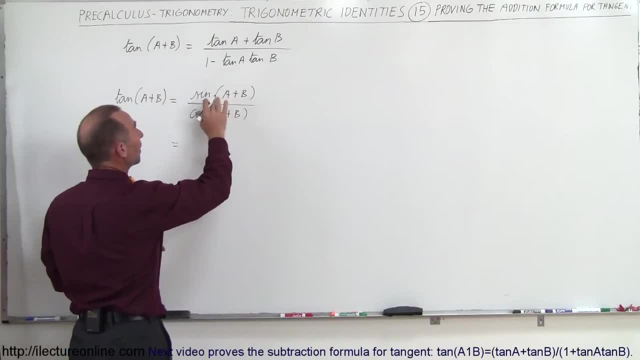 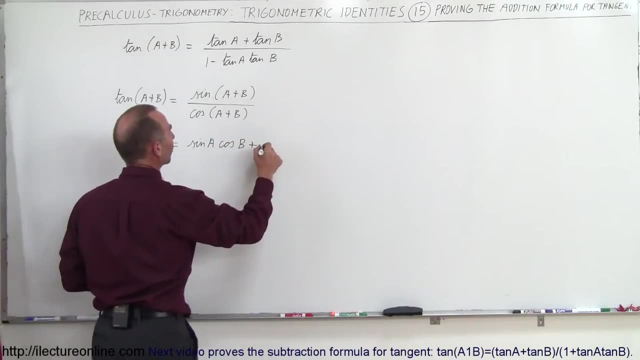 in the right direction. So this is going to be equal to the sum of a plus b for the sine. So that means we have the sine of a times the cosine of b plus the cosine of a times the sine of b divided by. and the cosine of a plus b becomes the cosine of a times the. 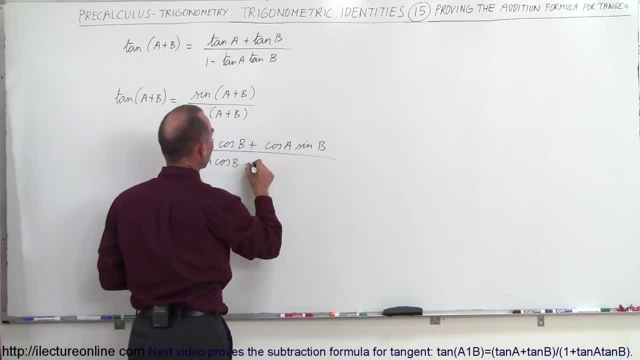 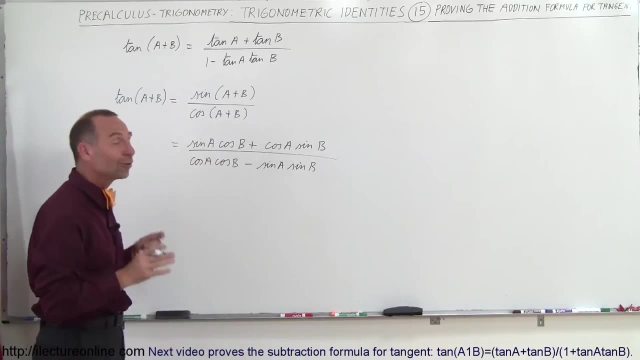 cosine of b, And that would then be minus the sine of a times the sine of b. Now this is where most people get stuck, because if you don't know the trick, it's very difficult to go on from here. But remember, you need to end up with a 1 here somehow. So somehow we need to turn. 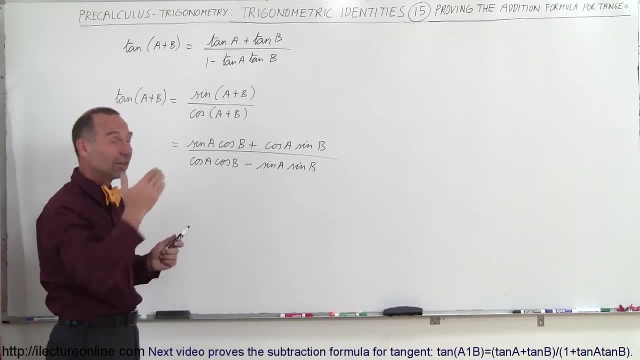 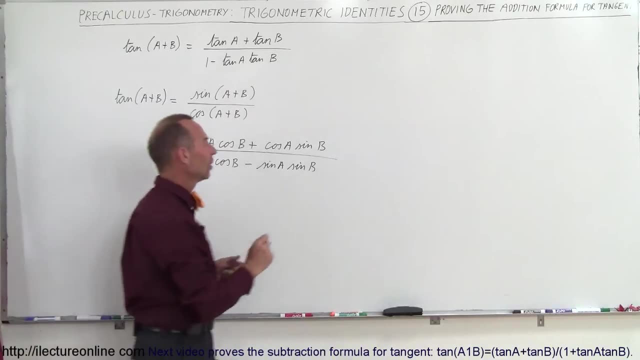 this into 1.. So that means, if we divide the numerator and the denominator by the cosine of a times the cosine of b, we can make this turn into a 1.. So that will give us that kind of gives us the hint. So this is going to be times 1 over the cosine of a plus b. 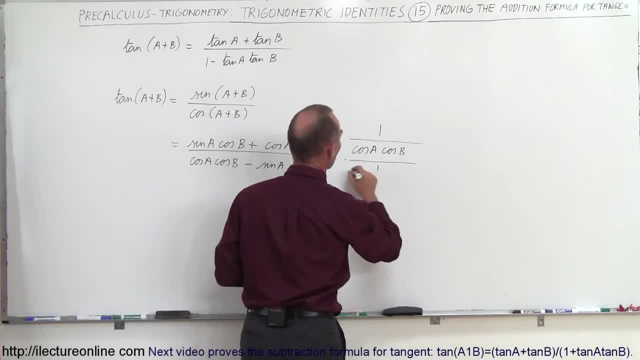 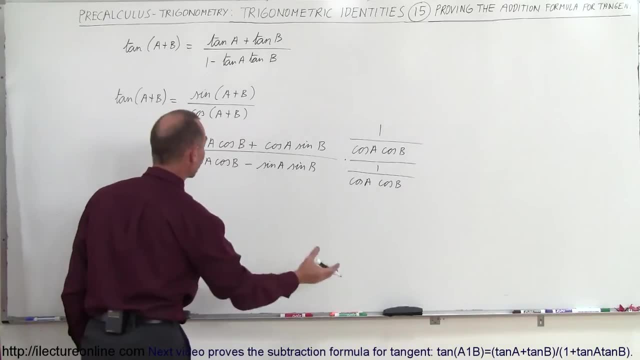 The sine of a times the cosine of b, divided by 1, over the cosine of a times the cosine of b. Now, hopefully, everything else will fall into place when we do that. So let's go ahead and multiply that through, So that gives us the sine of a times the cosine of. 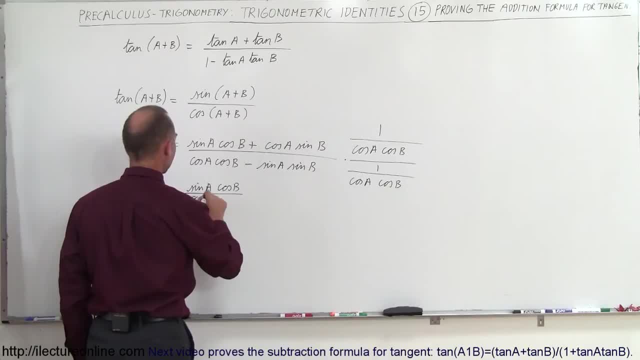 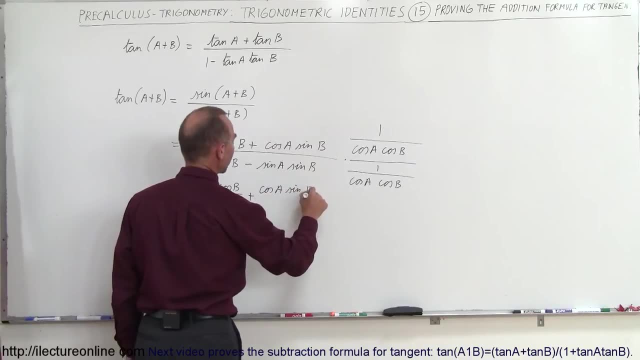 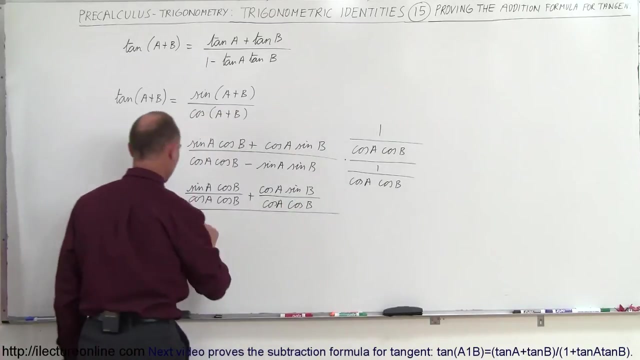 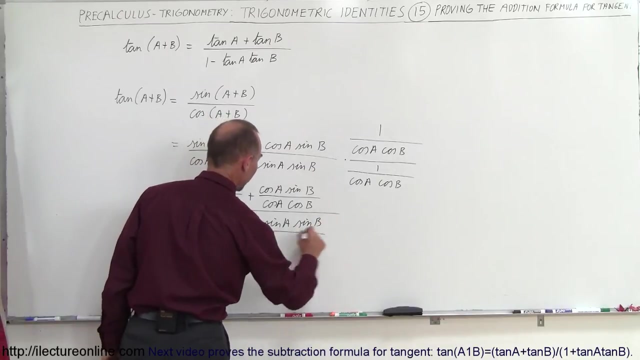 b divided by the cosine of a times the cosine of b, plus cosine a sine b divided by cosine A cosine B, And the whole thing divided by. we have cosine A cosine B divided by cosine A cosine B, and that will give us the 1 minus sine A, sine B, divided by cosine A cosine B. 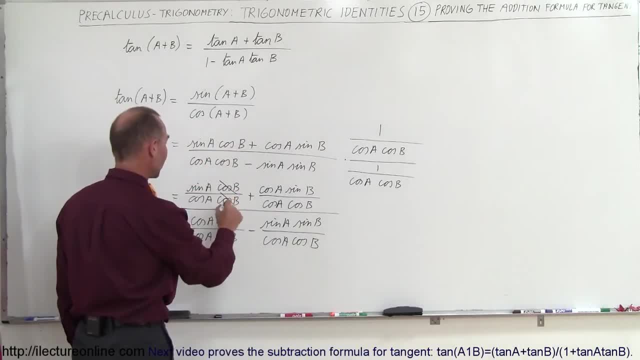 Alright, let's see what simplifies. So here we have cosine B, cosine B, we have cosine A, cosine A. This whole thing turns into 1, so let's see what we get when we do that. So this is equal to sine A divided by cosine A, plus sine B divided by cosine B, all divided.